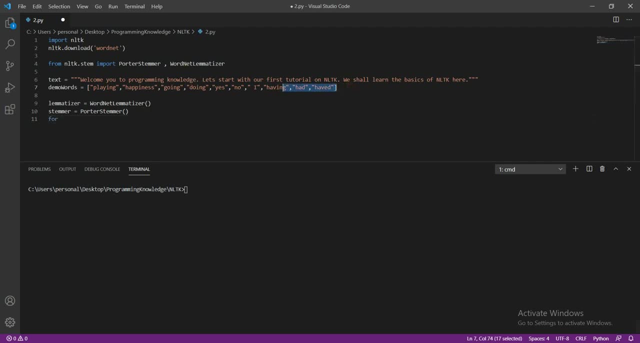 Here you can see, Okay. So what we can do, we can type for word in demo words, Okay, And like we can do in, We can do in stemmer dot. stem word, Okay. And we can do lemmatizer- lemmatizer dot. lemmatize word. comma p. 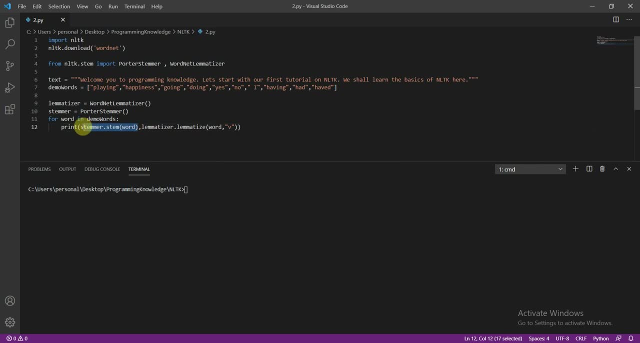 So this is just like. these are two like stemmer dot- stem word and lemmatizer dot- lemmatize word, And we stand for verb. So basically what we are doing, I'll explain you in short. Just wanted to have a quick overview of the coding part. 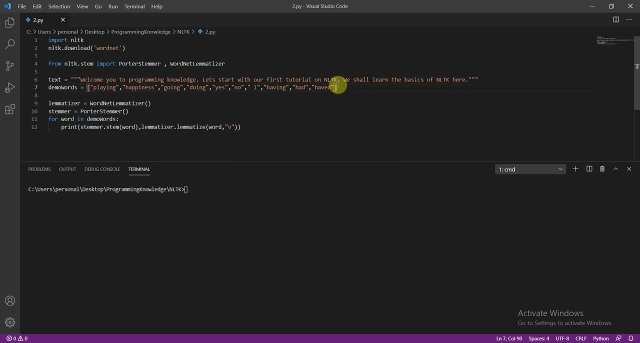 Now I'll focus what this stemming and lemmatization does. So let's add some Python like random words, like coding programming, Okay, Code program, something like this: Okay. So in the left we have Like: left is step in left. 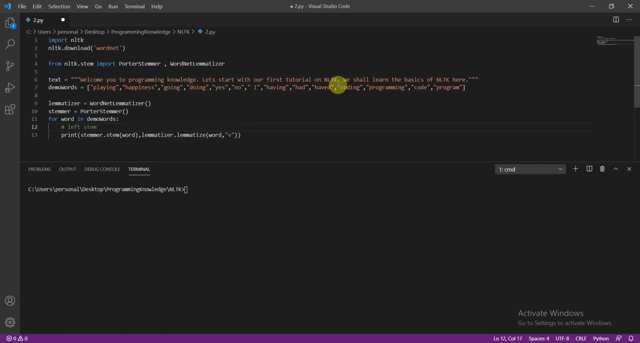 We had the stemmer. Okay, Left is the stem And in right we have. the right is we have the lemmatize. Okay, Okay, So this is how we do So. like this. Let's run this file, Oh yeah. 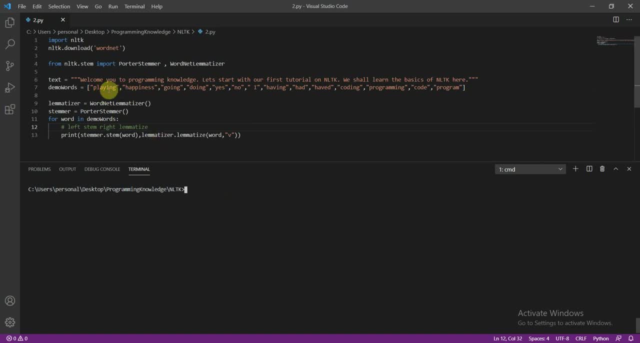 So what we are going to tell that? basically it converts all the verbs. like we already know, the verbs have already the like: some are in present tense, some are in past tense, present Future and Past, Past present- something we all, we there are, on different forms. 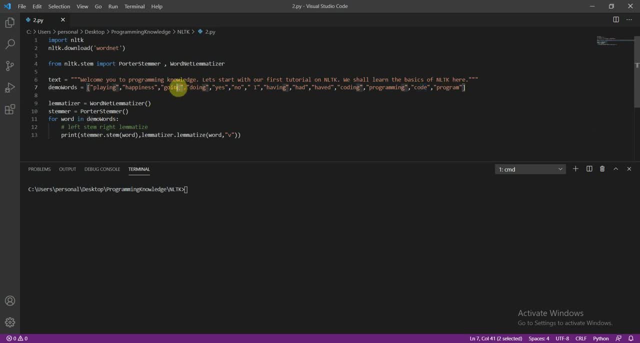 So we can say: playing, happiness, Going, doing, yes, No, I have having, have, basically having, and have coding programming, a Koda programme or basically already related to each other, like going or doing, are similar to go. Okay, And we are w we know. 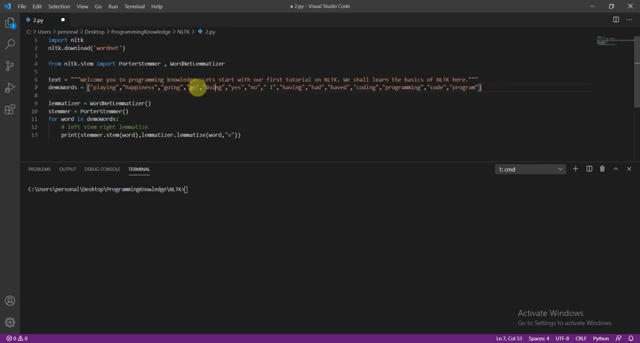 we know they are very similar. go and in the same way. doing is very similar to do. okay, so this is just a way of converting them into their original raw form instead of the verb form. they are existing, which could be present past something. so let's run this file, so here you can see. 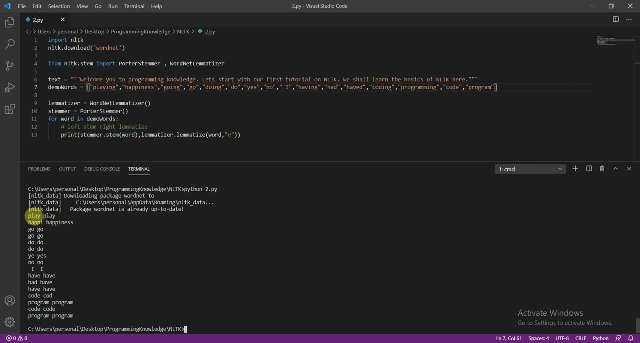 so here you can see that play is converted to this. okay, let me do also print the original word. okay, so this is how we do. so we have the order would be: this would be the word them and limitize: okay, and now let's run this again. i'll remove this. yeah, so let's run this. so we see. we see the. 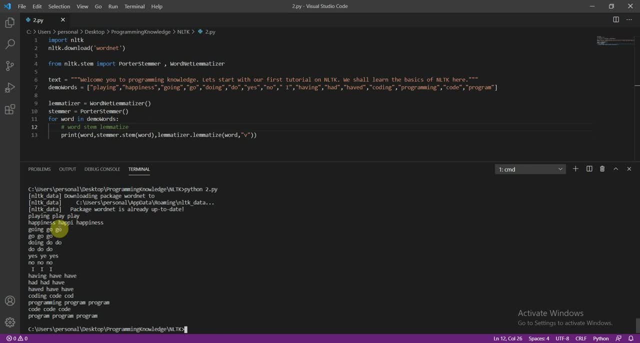 word playing is converted to play. happiness is converted to happy happiness. going to go, go, go go is already doing to do and do. okay, both of them convert to do and yes to yeah, yes, no. i having is converted to have, have this converted to have, because having or have meant the same thing their original form was, have had is converted. 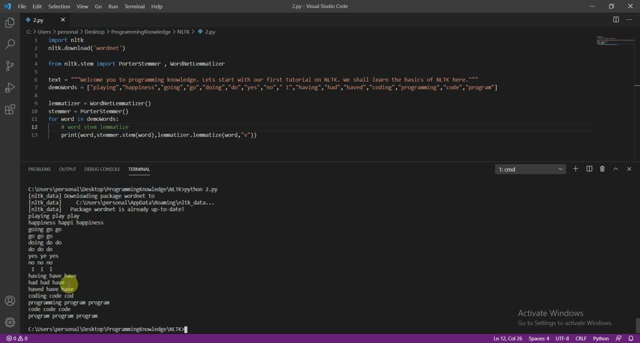 to had and have okay. so basically, uh, you can see with context, the lemmatization uh is more accurate okay than stemming. so basically both of them do the same work. programming is converted to program and uh, programs is same and coding is converted to code and code. so basically, uh, in some context, but uh. 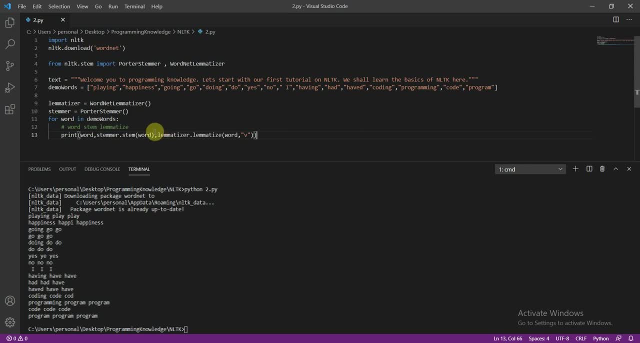 uh like. both have their own advantages and disadvantages. but looking at that, like, uh, we can say that, uh like, since some sense of stem, stemmer, stemmer is accurate, but lemmatization is accurate, but the both of them have to like, uh like. it all depends. 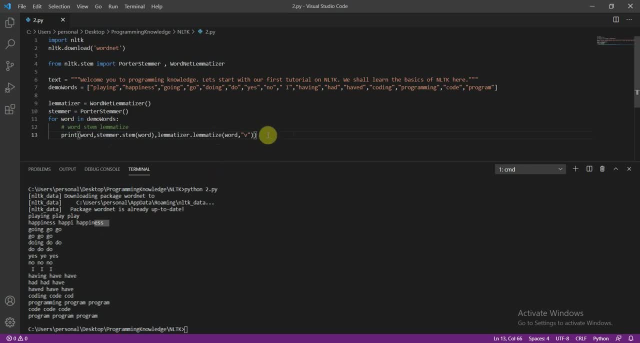 on you that which result has a better accuracy. but both of them do the same: that they convert all the uh verbs into their original form. so this is how we deal. okay, so this is the way we deal with uh, lemmatization and stemmer. so let's comment this. now let's move to the another. 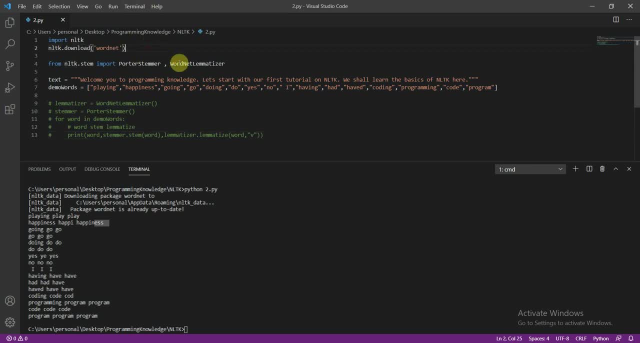 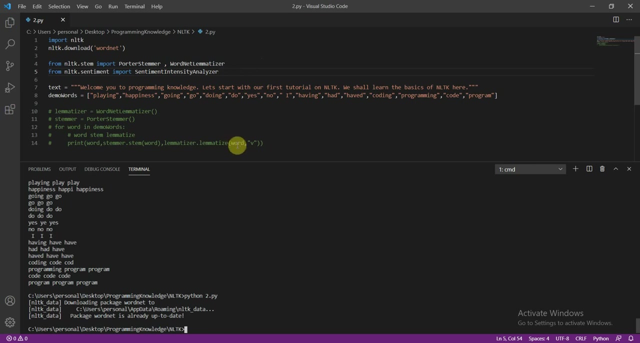 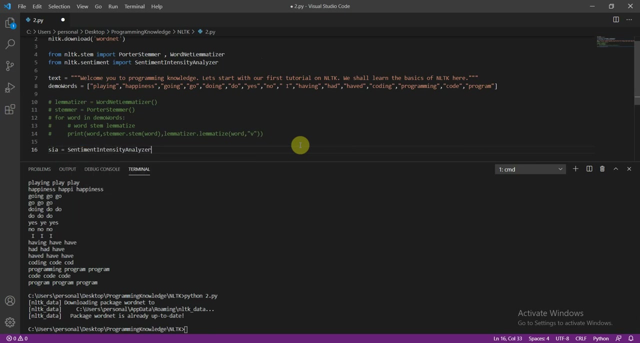 one. uh, we can do from nltk, nltk, nltk, dot. sentiment import- okay. so let's create a sentiment intensity analyzer, let's write an object called sentiment sentiment sentiment intensity analyzer- okay, and let's run this file to make sure that this is going in the right direction. so yeah, so we are like, uh, in right direction. 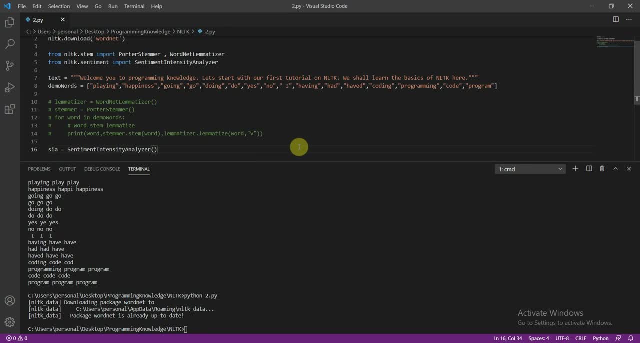 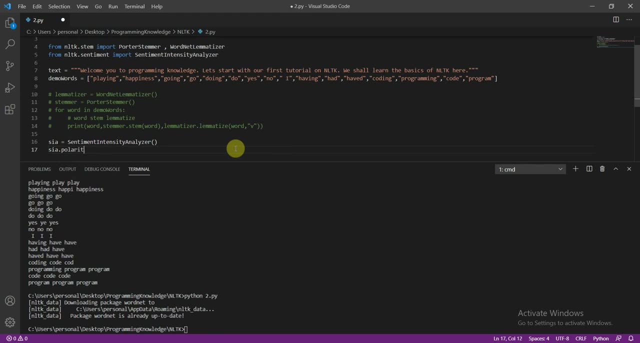 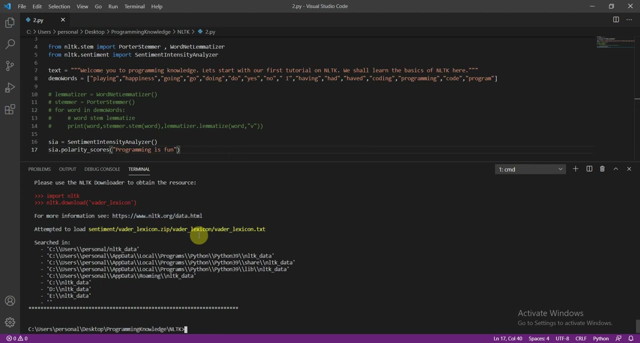 initialize this class and what we can do. I can do si a dot, polarity, polarity, underscore scores. so these are three scores which is going to be defined and we need to find the sentence. so I'll define programming this one again. when I run this here, you can see, I'll clear this. yeah, when I run this here, you can. 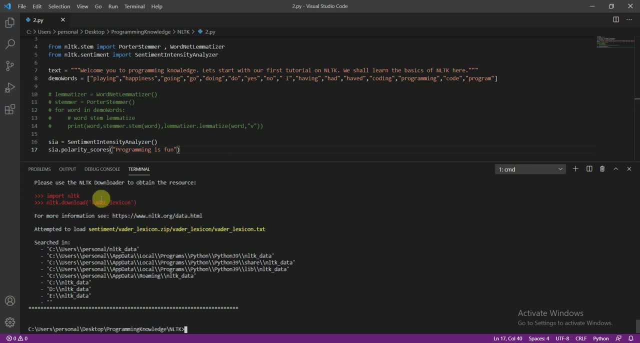 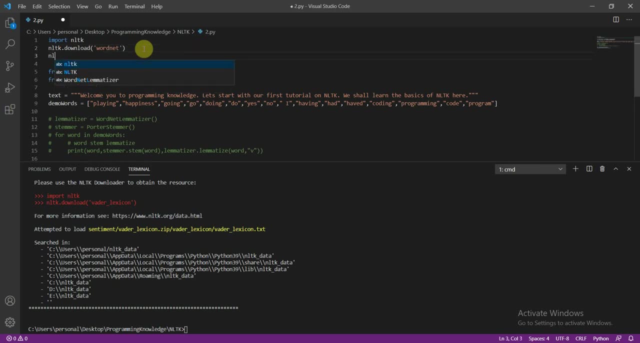 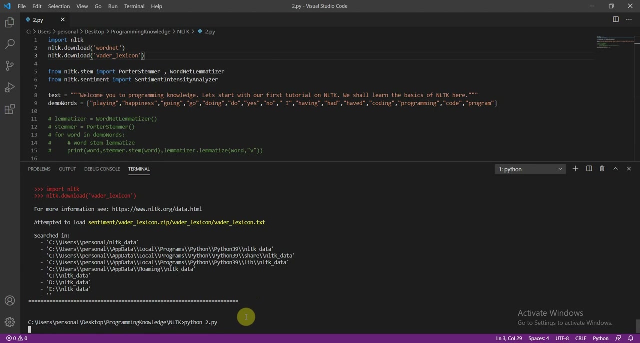 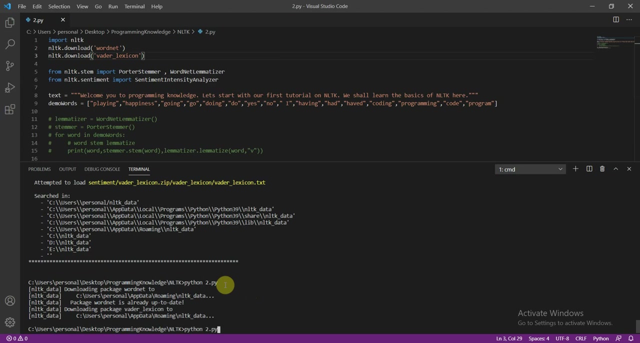 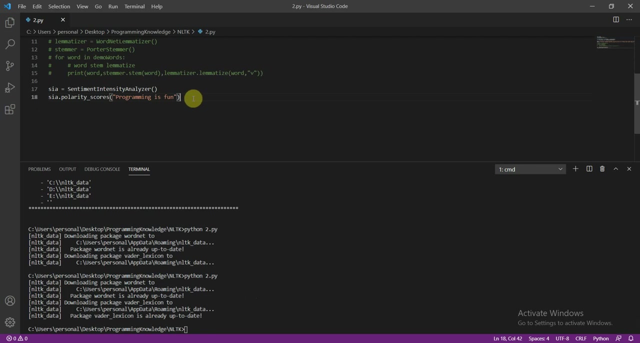 see, okay, this is waiter and the whole lexicon is not installed, so we can change. okay, also, NLT K dot download: waiter, waiter underscore lexicon. okay, okay, and now let's run this file. so ok, I had run this, ok, ok, ok, ok. yeah, I made a mistake that I had to print this statement. 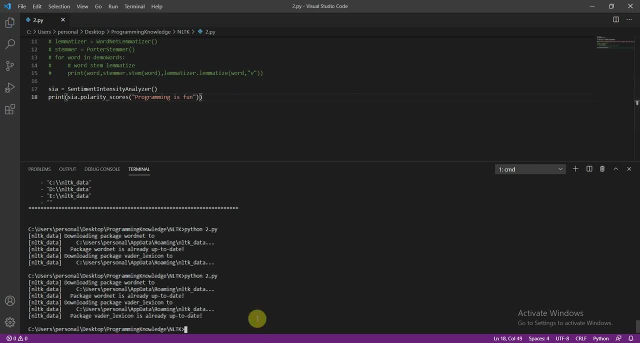 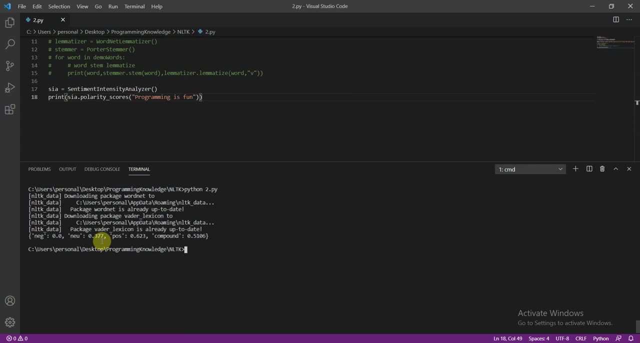 so that's why it wasn't printing. so let's run this again. yeah, now you can see. so it says negative score is 0,, neutral is 0.377 and positive is 0.623. this is a positive statement, so you can make a logic that which one is maximum you can assign it to that.